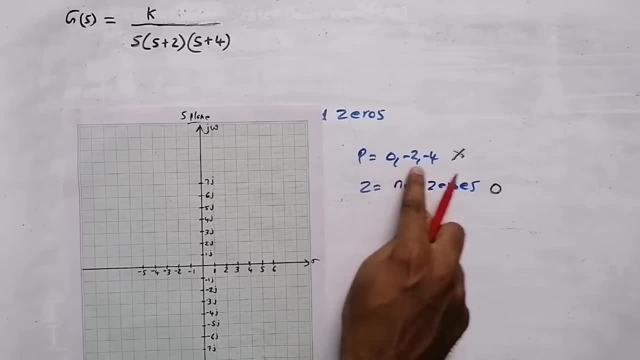 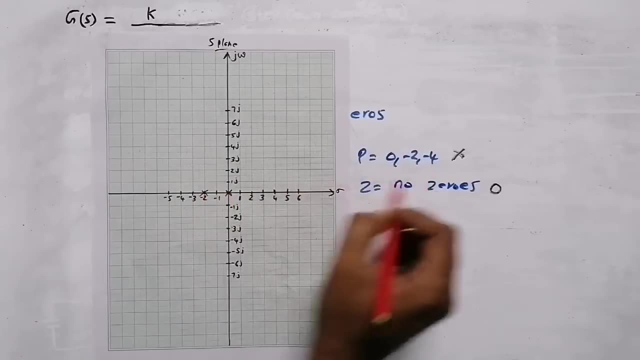 Now I am going to plot poles. First of all I am going to plot poles. So poles are at zero, minus 2 and minus 4.. Zero, So here there is one pole, Then at minus 2.. Minus 2 there is a pole and minus 4. Minus 4 also. 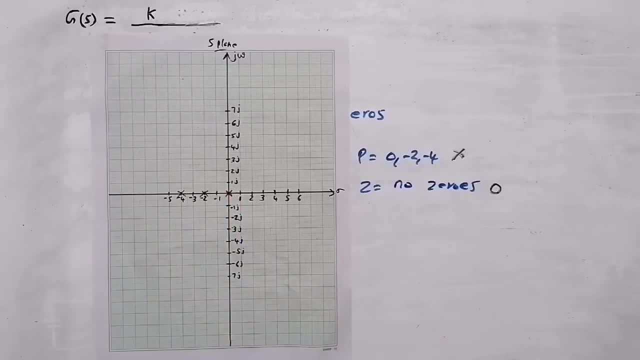 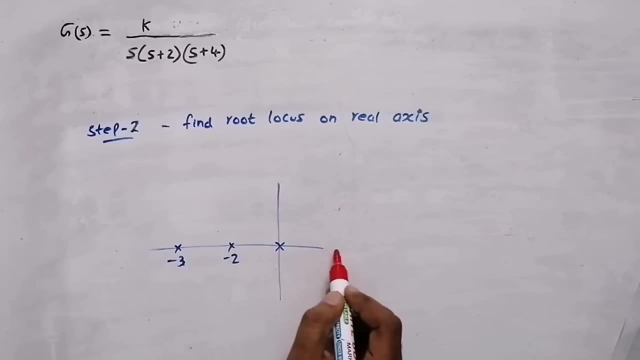 there is a pole, So these are the number of poles. In this case there is no zero. So after plotting poles on the graph sheet, now we have step 2, to find root blockers on the real axis. So this is our real axis. We need to find root blockers For that. 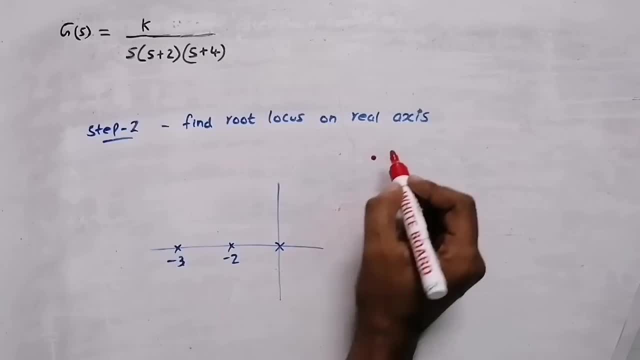 I need to use a test point. So when I use a test point here, if I am getting odd number of poles and zeros on the right side, then root blockers will be existing. If I am getting even number of poles or zeros, then root blockers will not be existing. 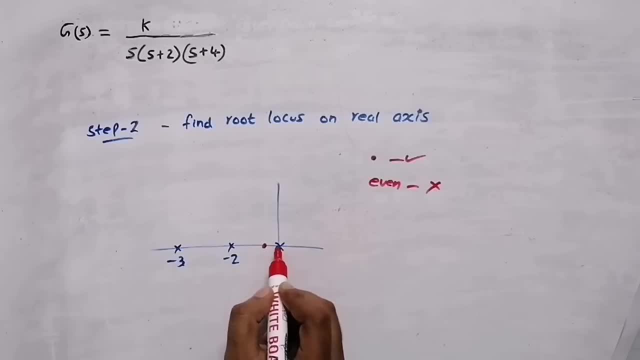 So my test point is here. Then I am checking: on my right side There is only one pole, So odd number of pole. Then my root blockers will be existing Here. also, if I am taking this pole and on the right side of that there is only one pole, That is odd, So my root blockers will be existing here. 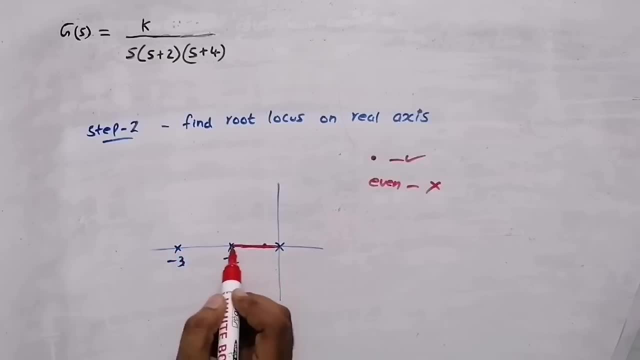 Then when I take this point, then there are even number. Two poles are there. That means even number. At that time my root locus will not be existing here. Then when I take a test point here, then I check 1,, 2,, 3.. 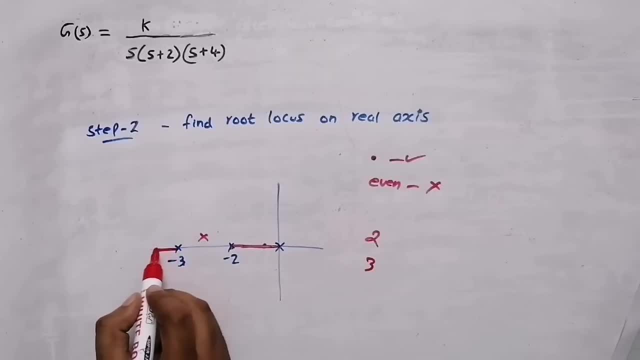 3 poles are there. that means odd number, So my root locus will be existing here. So from poles, always root locus will start and either it will end at infinity or it will end at 0.. So root locus will start and it will go to infinity. 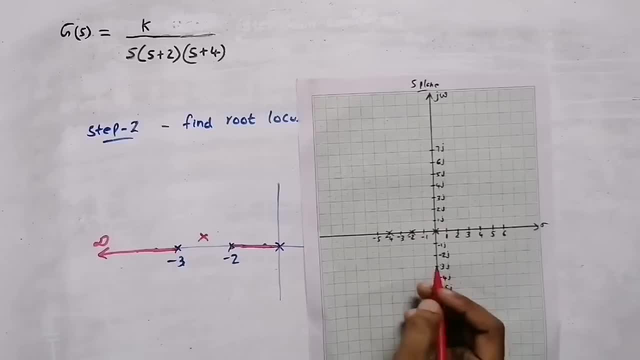 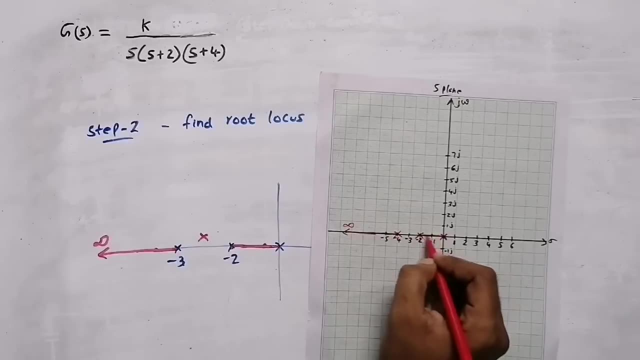 Here there are no 0, so it will go to infinity. So in the graph sheet, my root locus will be existing here and also to infinity. So in this region my root locus will be existing. Now we need to find asymptotes and centroid. 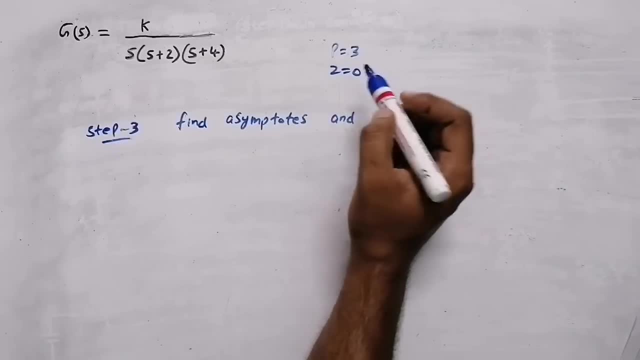 Here there are 3 poles, We have 3 poles and 0s, we have 0. So there are 3 poles, so there will be 3 asymptotes. Asymptotes are just straight lines. They are just straight lines. 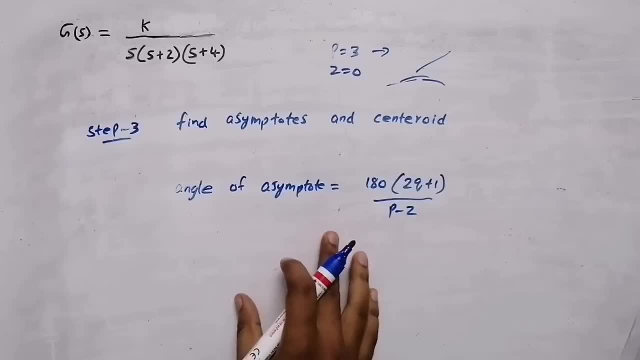 And for finding asymptotes. we need angle of asymptotes. For getting angle of asymptote, this is the equation: 190 into 2q plus 1 divided by p minus z. p is number of poles and z is 0.. 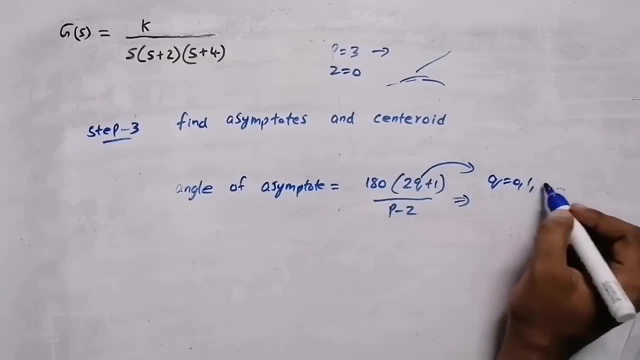 So where q, q is 0., 1. Up to p minus z minus 1.. So in this case the angle of asymptotes will be 180 into 2q plus 1. divided by p minus z, p is 3.. 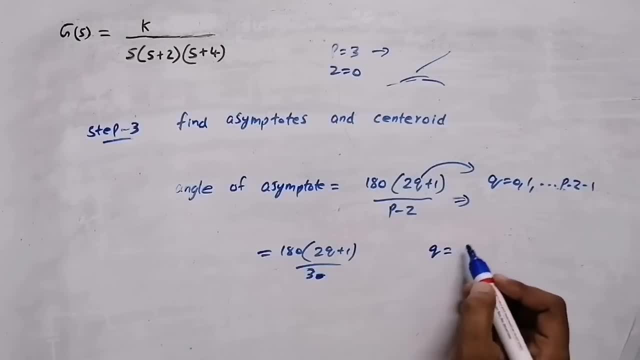 3 minus 0.. That will be 3 itself. Okay, So our values of q will be 0, 1 and p minus z minus 1.. p minus z, it is 3.. 3 minus 1, it will be 2.. 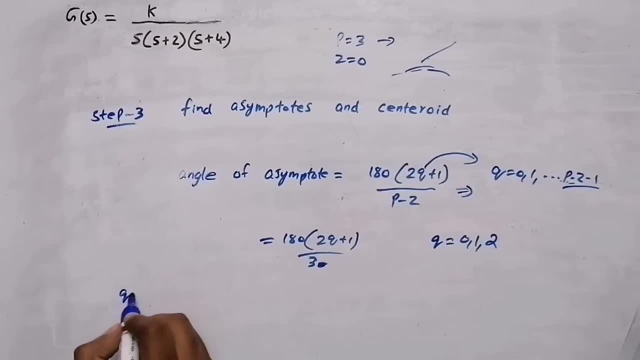 So the values of q will be 0,, 1 and 2.. So when we have q equal to 0,, our angle of asymptote will be 180 into 2, into 0. It will be 0.. 0 plus 1, it will be 1.. 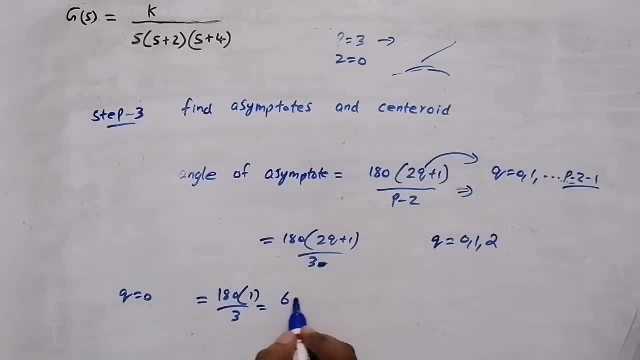 So 1 into 180 by 3. That will be equal to 60 degree. Then when we have q equal to 1, our equation: 2 into 1, it will be 2.. 2 plus 1, it will be 3.. 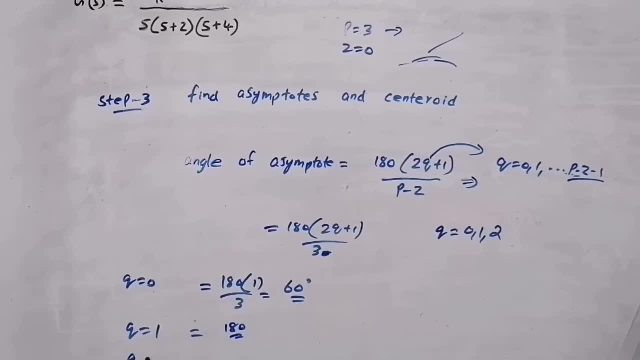 So 3 and 3 will be cancelled. We will get 180 degree. Then when we substitute q equal to 2, then it will be 180 into 2 into 2, it is 4.. 4 plus 1 divided by 3.. 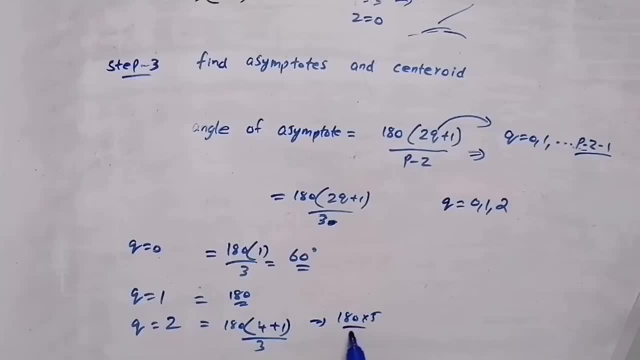 So 4 plus 1, it is 5.. So 180 into 5 by 3. 3, it will be 6.. 60 into 5, it will be 300.. So the angle of asymptotes are 60 degree, 180 degree and 300 degree. 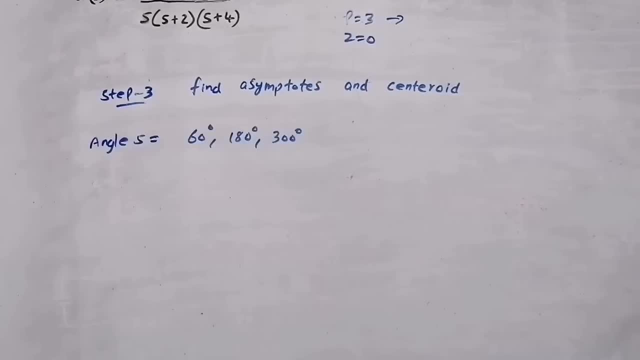 So number of poles is 3.. So there will be 3 asymptotes. Now we got the angles for asymptote. Now we need centroid From where these angles will start. Okay, For that we need centroid. How to find centroid? 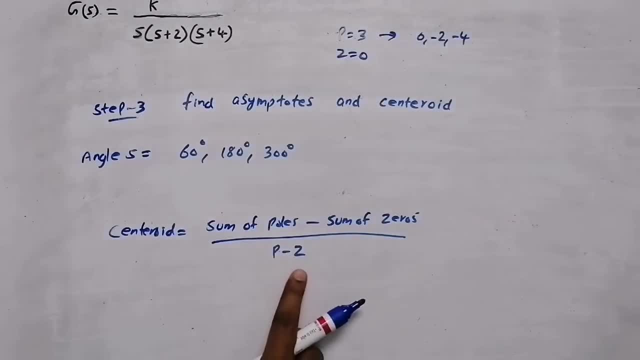 Centroid. the equation is sum of pole minus sum of zeros divided by p minus z, Sum of poles. For poles are 0, minus 2 and minus 4.. 0, minus 2, minus 4, minus sum of zeros. 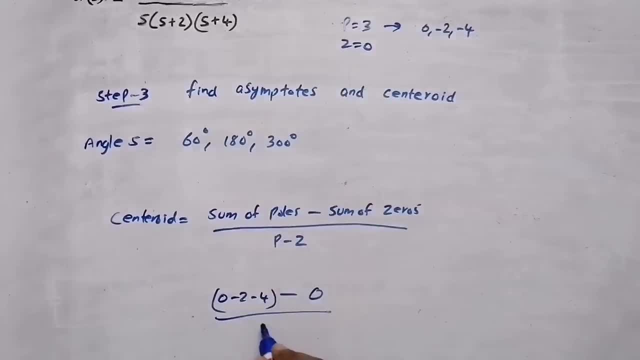 There are no zeros. Divided by p minus z, p is 3, number of poles and number of zeros: it is 0. So minus 2, minus 4, it will be minus 6 divided by 3. Then you will get us minus 2.. 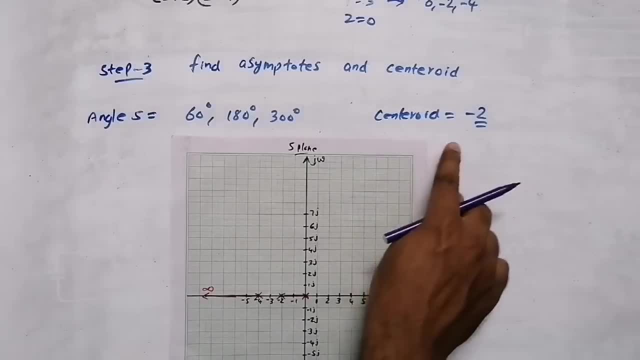 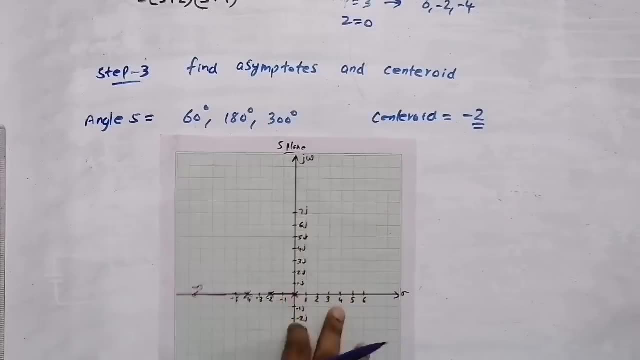 So centroid will be at minus 2.. So at minus 2, we will have our centroid. Now, after finding centroid, we need to plot this angle: Centroid is at minus 2.. For minus 2, we need to plot 60,, 180 and 300 using protractor. 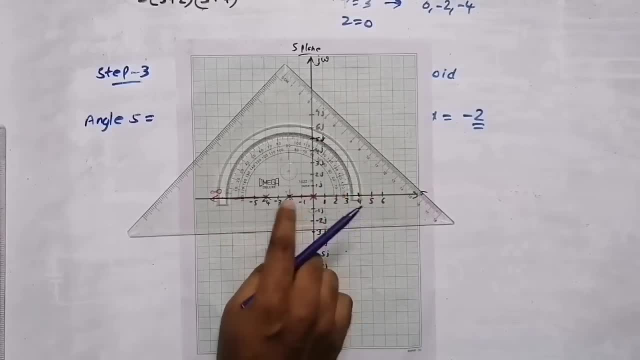 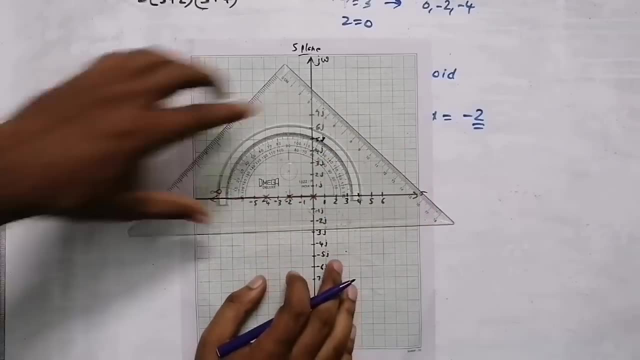 So first of all we can plot minus 60 from point minus 2.. Minus 2, we need to take the center, Then plot 60 degree, Then 180 degree, Then for plotting 300 degree, either you can rotate the protractor or you can. 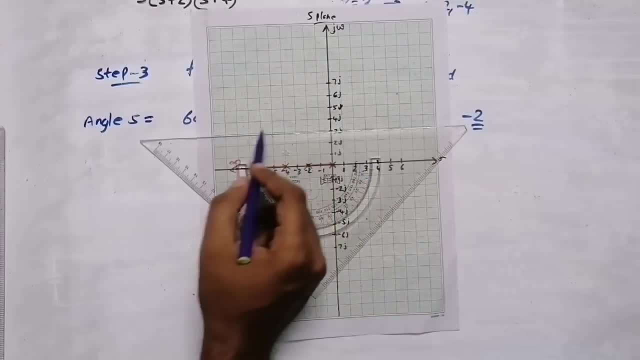 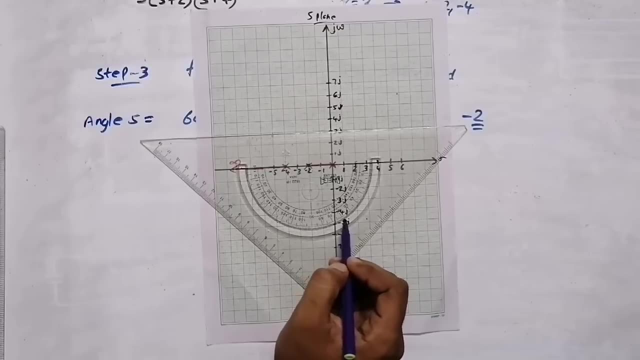 or you can take. So if I am rotating the protractor from here, I am getting 0, 180, then 270, then 300. That is minus 60, 300.. Okay, Minus 60. Then it will be 360. 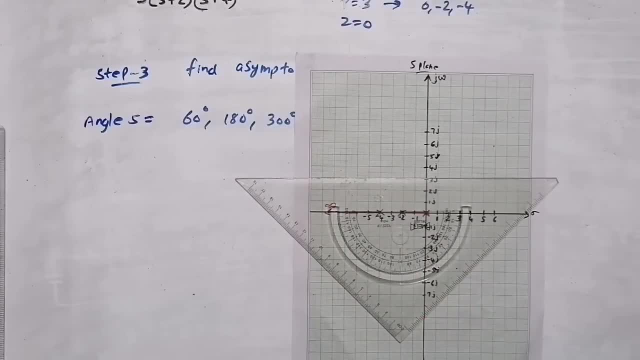 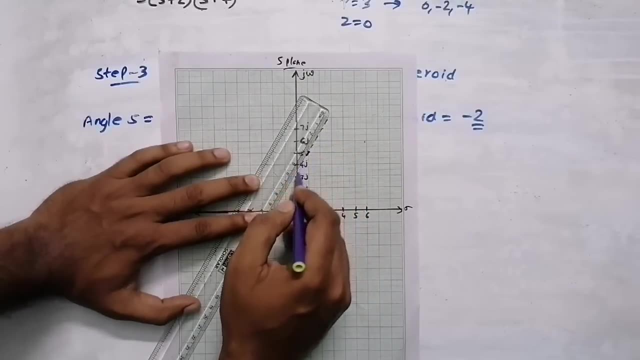 So my three angles are 60, 180 and 300.. I need to plot these angles. Now, asymptotes: you need to draw with dotted lines. Okay, Dotted lines, They are just straight lines. So use a scale and draw dotted lines from the centroid. 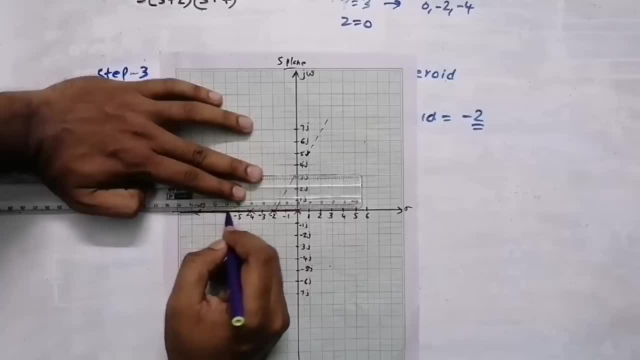 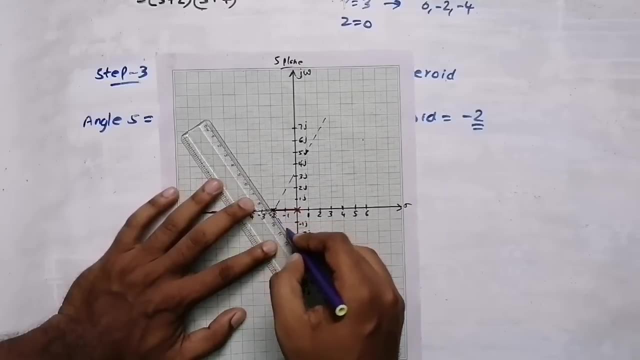 So one is at minus 60. Then 180. And the other one is at 300, or you can take minus 60, 300, or you can take minus 60. So these are my three asymptotes, asymptotes you always. you need to draw with dotted lines. 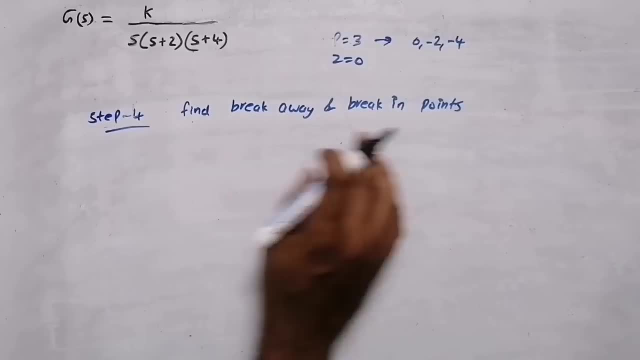 Now in step four, I need to find breakaway and break in point. So, as I said earlier, always root local cells start from pole and end at either zero or it would end at infinity. So when there are adjacent poles it will start from pole. 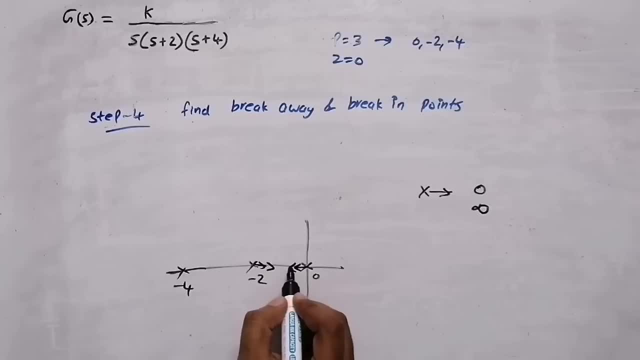 It will start from pole. Here also it will start from pole, but we need to know. we need to know where it will meet. At a point It will meet. We need to find that point. That point is breakaway. When there are adjacent poles, we will get breakaway. 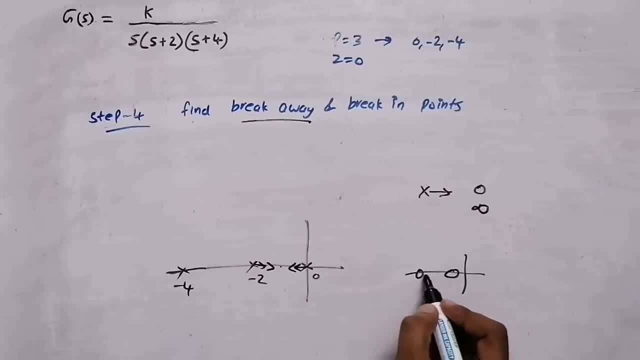 When there are adjacent zeros- and there are adjacent zeros always- the root lockers will come and end at zero. They will end at zero or infinity. They will end here. They will start, here They will end. So this arrow mark like this, here the arrow mark, it is like this: 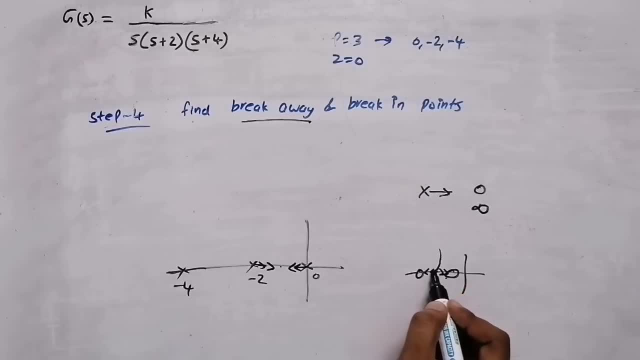 So at the point they will meet and end like this, from here it will come and end like this. So that meeting point we need to know that is break in, break in, This is break away. They're going away. This is break in. 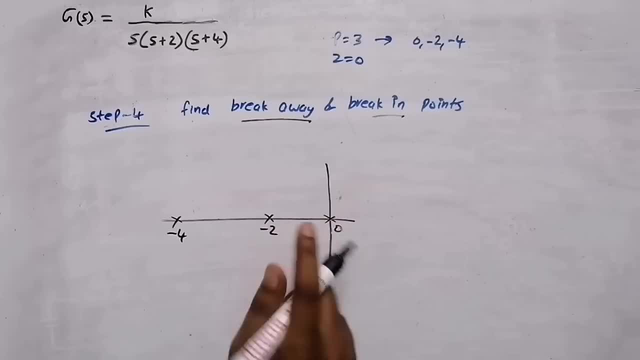 They're coming. So in our question we have two adjacent poles and our root lockers will start from pole and it will meet at some point. That is our breakaway point. We need to find that breakaway point. How to find it? 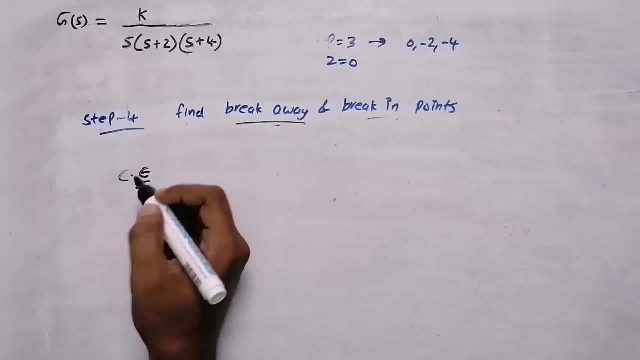 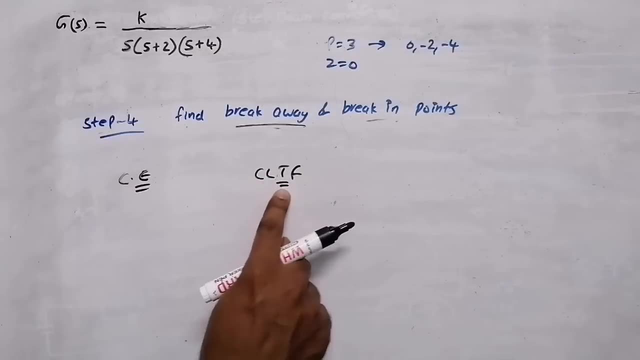 For finding breakaway or break in, we need to know characteristic equation. So how to get characteristic equation? We need to write the closed loop transfer function. This is open loop transfer function. From that we need to write closed loop transfer function. 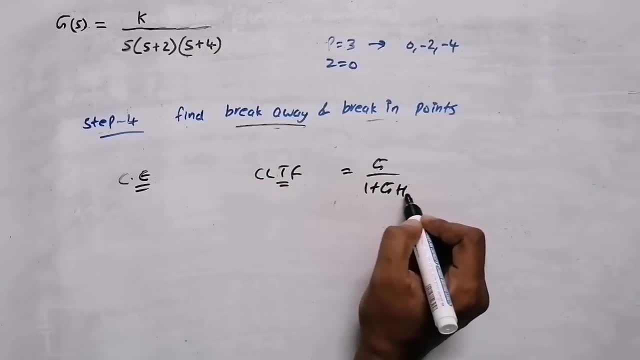 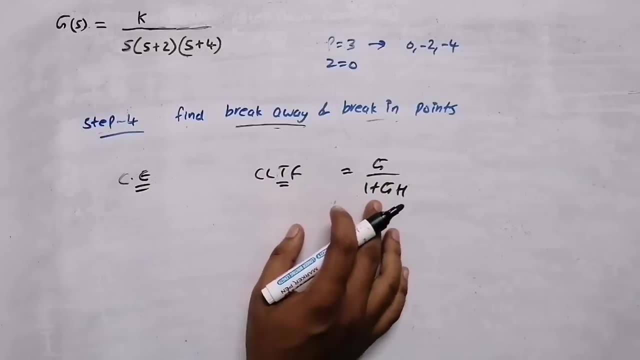 So how to write closed loop transfer function: g divided by one plus gh. If it is a negative feedback, if it is a positive feedback it will be one minus gh. But in this question nothing is mentioned, So you can take it as negative feedback and find g by one plus gh. 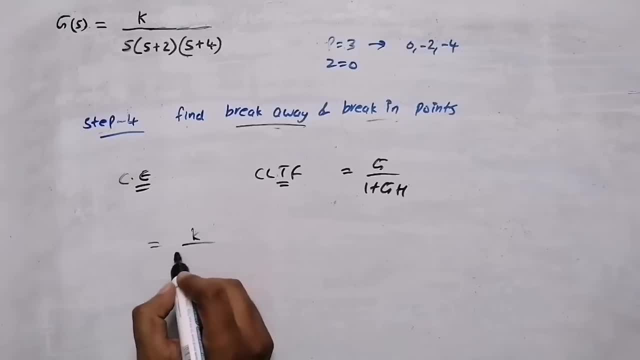 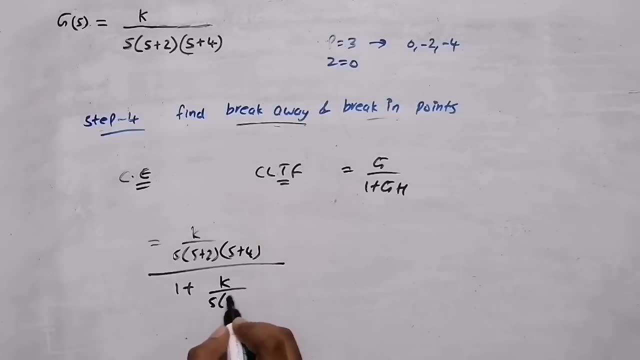 So what is our g? This big thing that is k divided by s, into s plus two, s plus four, or divided by one plus g. G is the same thing. Substitute it: S plus two, s plus four, Then h, it is unity, unity, feedback. 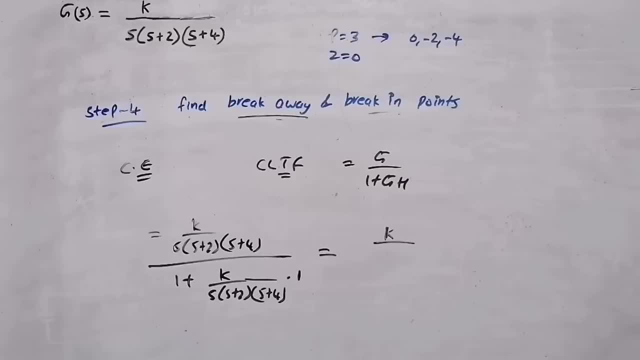 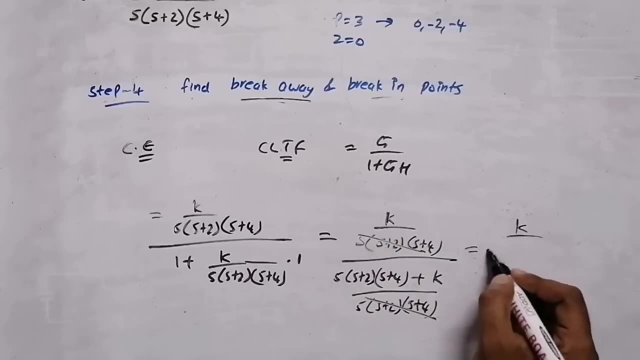 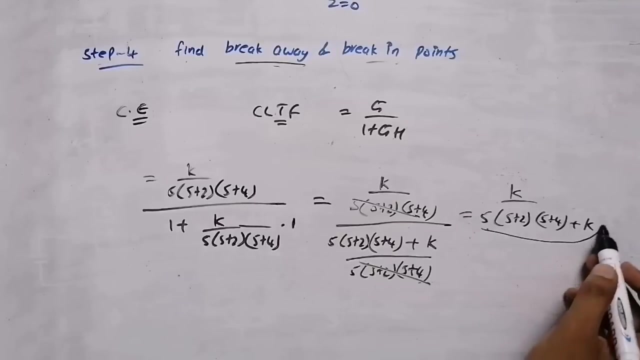 So h equal to one. Then, solving this, we will get by cos multiplying it. Okay, We will get. now, removing this denominator, we will get the final answers: k divided by one plus gh. Now we will get the characteristic equation when we equate denominator equal to zero. 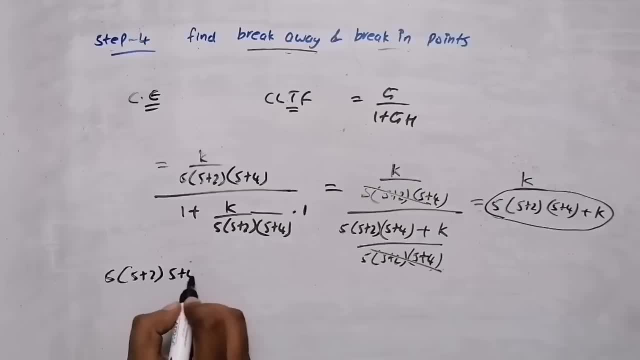 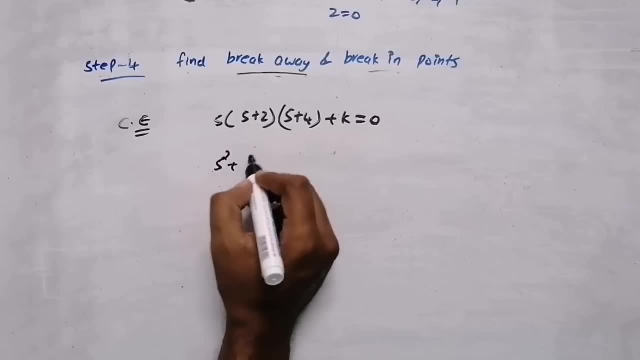 So what is our denominator? s into s plus two, into s plus four plus k, equal to zero. Now we need to expand the bracket, open the bracket, So s into s, it will be s square plus s into s and s into two. 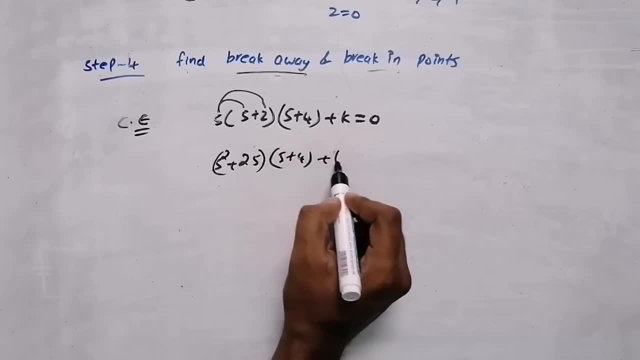 So s square plus two s into s plus four plus k, equal to zero. Now, s square into s, it will be s cube. s square into four, it will be four s square Plus Two. s square plus four into two, it will be eight s plus k, equal to zero. 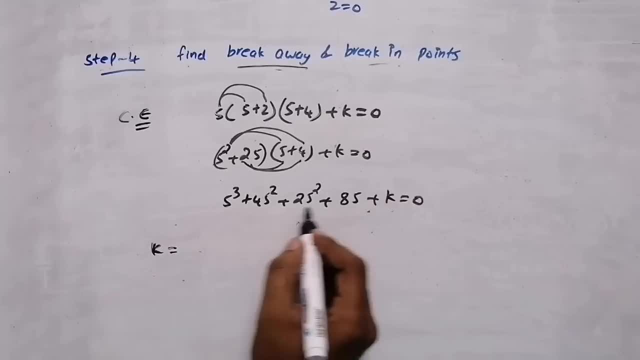 Now, from this equation, find the value of k From getting k what we need to put all this at the other side. So we will get minus s cube minus four plus two. four plus two, it is six. So we will get minus six x square minus eight s. 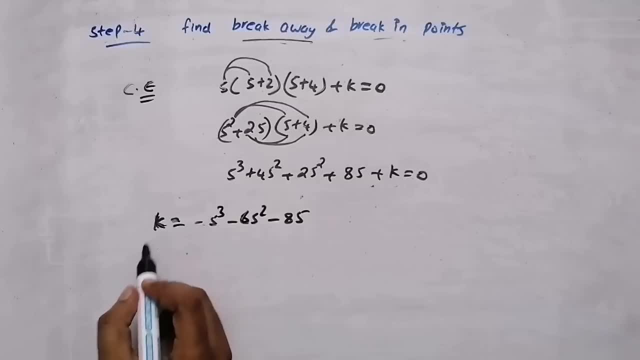 So this would be our k. Now differentiate this and equate it to zero. dk by ds equal to zero. Differentiate this equation and equate it to zero. So, differentiating it, we will get three s square Minus minus three s square minus twelve s minus eight. 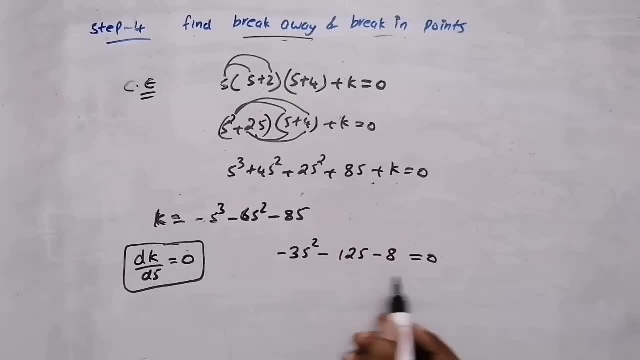 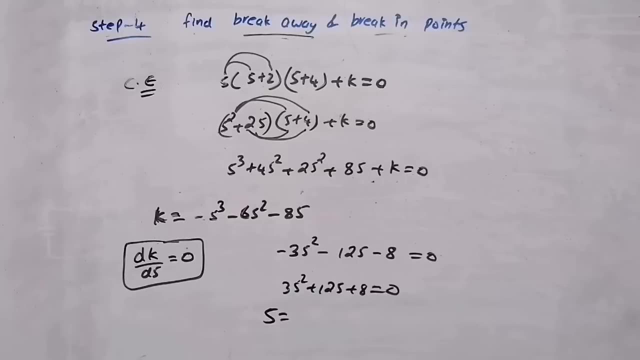 Now, equating it to zero, we will get. we can take the minus outside and equate it to zero, We will get three s square plus twelve s plus eight, equal to zero. From this we need to find the value of s by using calculator. 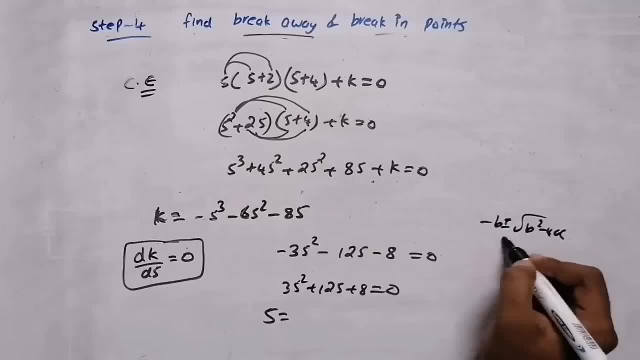 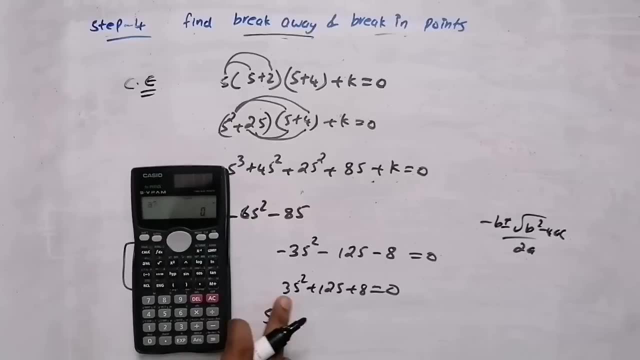 Or you can use minus b, plus or minus root of b square minus four s c by two a. That equation also you can use, But I am using calculator equation. This is second degree equation. So two, The coefficient, here, at s square it is three, then twelve, then eight. 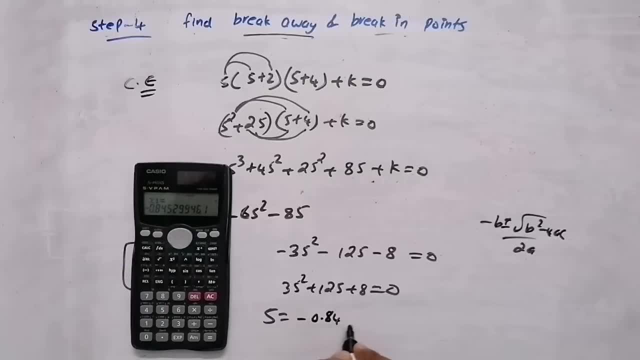 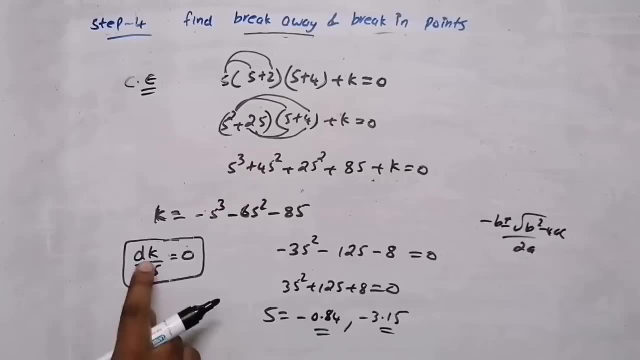 We will get the value as x one. it is just minus point eight four, then x two. it is at minus three point one five. So these are the two points that I am getting when we substitute dk by ds equal to zero. Now we have two points. 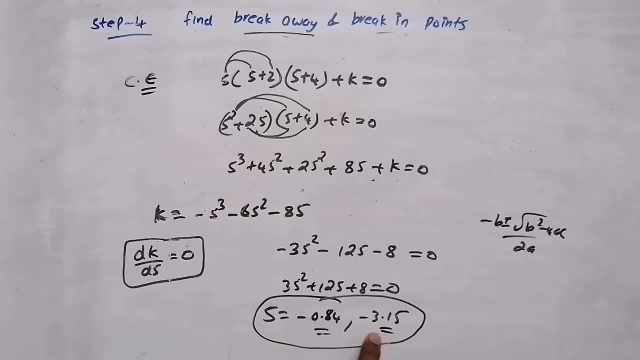 So these are my breakaway points, But there are two points. I need to find which point is existing. Okay, Which point is my actual breakaway For that? take my graph. There are two methods. Either you can use these two methods. 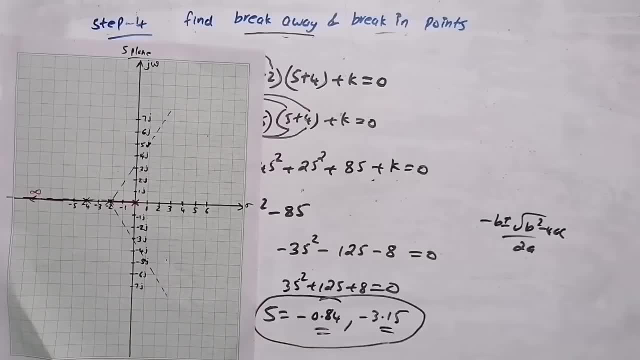 First method check. this point s is minus point eight four, Minus point eight four. it is lying. it may be lying here, Minus one is here. So minus eight point, minus point eight will be lying at this point. 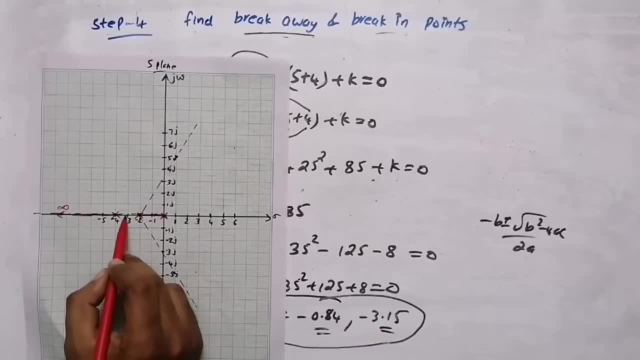 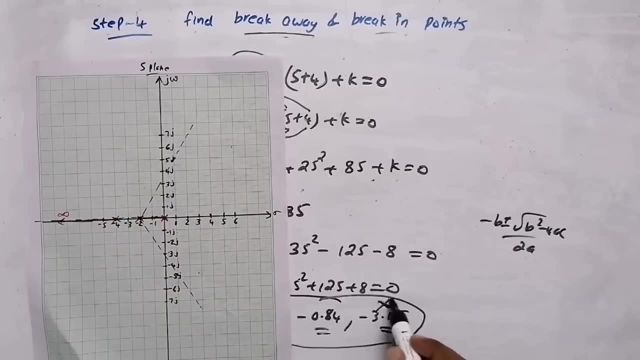 Then minus three point one five. minus three, minus three here. Minus three point one. five is here, But at this point the root locus is not existing, So this will not be my answer. My answer will be: minus point eight four. 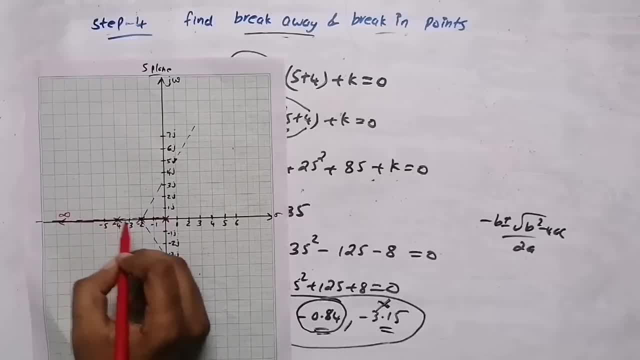 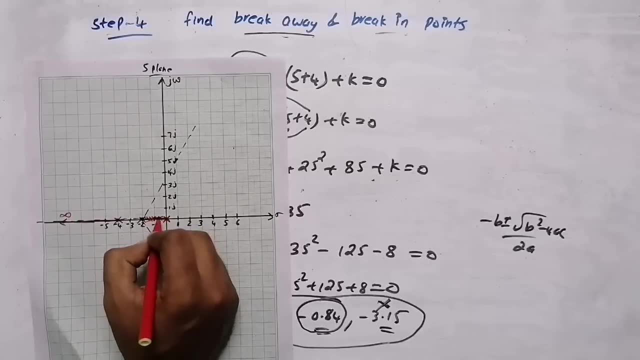 Because my root locus will be existing here and here. Here my root locus is not existing. So minus point eight four will be my breakaway point. So my poles will start and it will meet here And from here it will break away. The other method that we can use is that. look at this equation k: 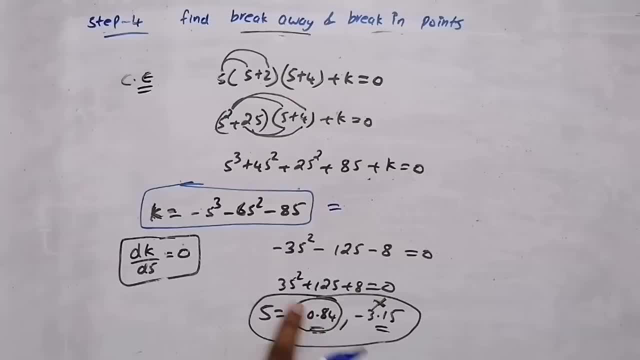 Substitute this value for s here. When we substitute s equal to 0.84, here we will get the answer as 3.08.. When we substitute minus 3.15 in this equation, we will get the answer as minus 3.08.. 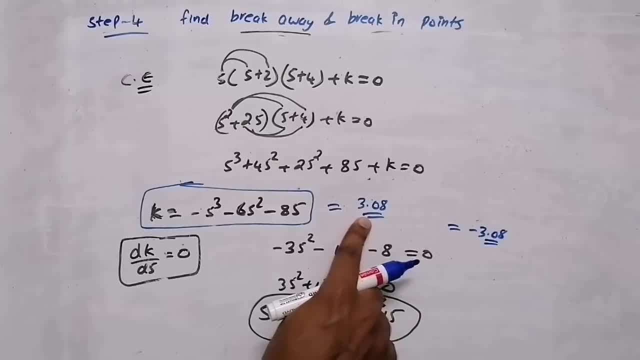 We are getting a negative value Always. we need to get a positive value for k. when we substitute our root, We will get two answers. When we substitute this answer in our k, we need to get a positive value. Then that value will be our correct answer. 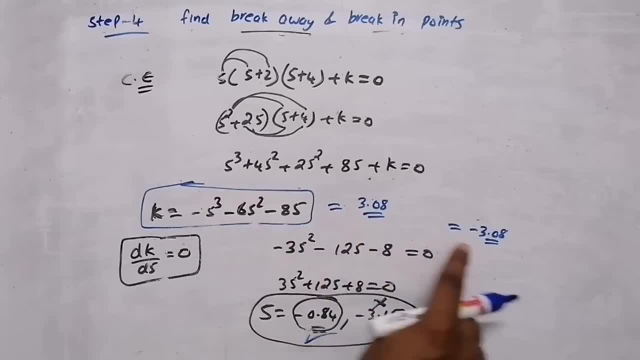 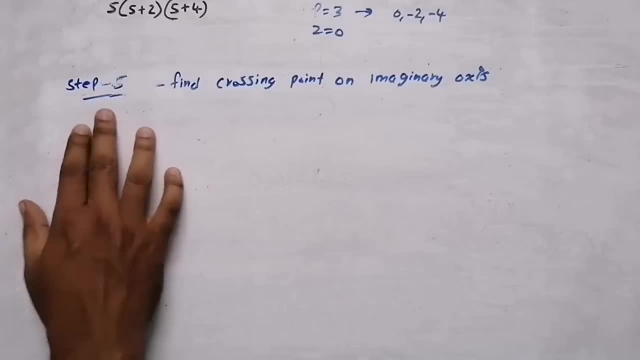 When we put this point here, we will get a negative value. That will be wrong. So this will be our breakaway point. Now, in next step, we need to find the crossing point on imaginary axis. So this will be our imaginary axis. 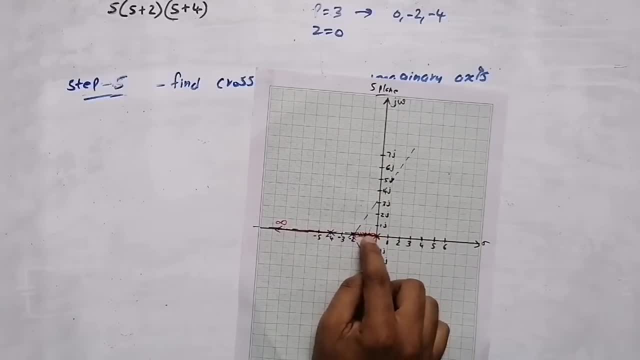 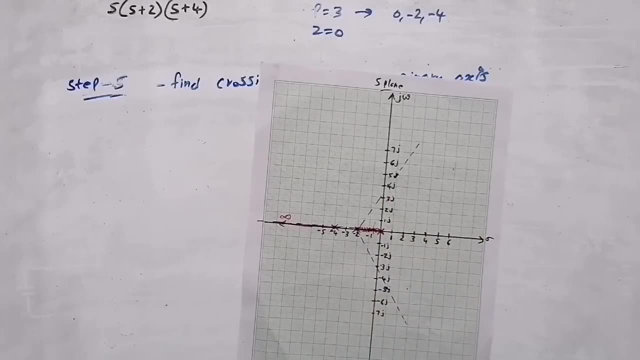 Our root locus will start from here and it will break away at this point And it will move like this. Then it will cross the imaginary axis at some point. We need to find that point where they are going to cross, For that from the previous step we got the characteristic equation. 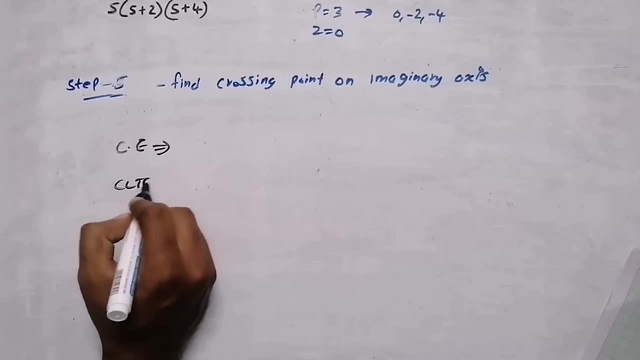 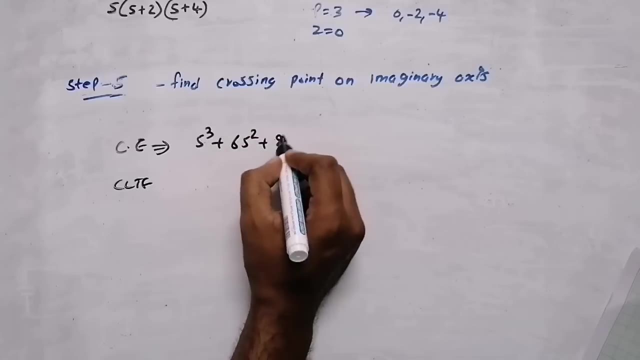 How we found the characteristic equation. We wrote the clause 2.. We wrote the function And we found the characteristic equation by equation denominator equal to 0.. So we get the characteristic equation as s cube plus 6s square plus 8s plus k, equal to 0.. 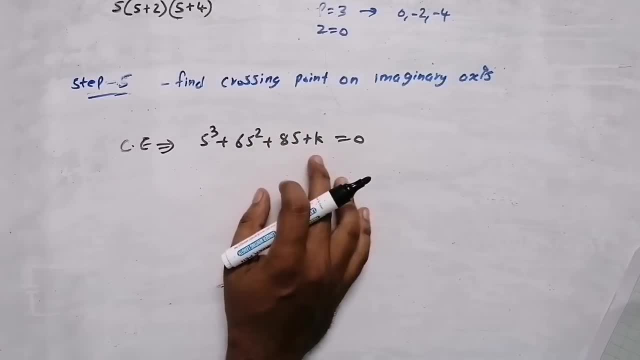 Now to find the crossing point from this characteristic equation: either you can use Ruth Hurwitz stability criteria or substitute j omega in this s Wherever you are seeing s you need to substitute j omega, But I am using Ruth Hurwitz. 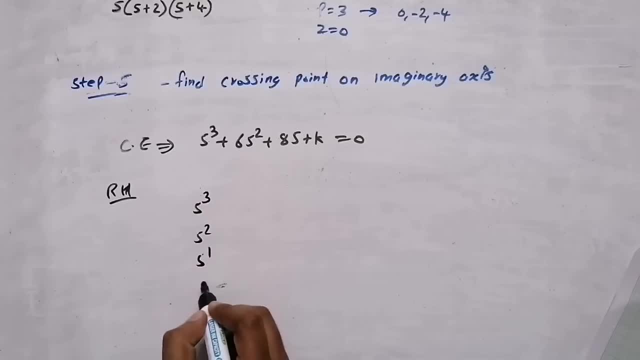 So first of all write the coefficient s cube, s square s raised to 1 and s raised to 0.. s cube, the coefficient is 1.. Then the alternate coefficient is 8.. Then here it is 6 and k. Now do the multiplication. 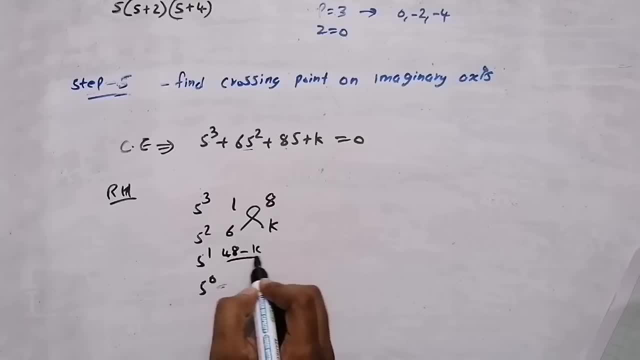 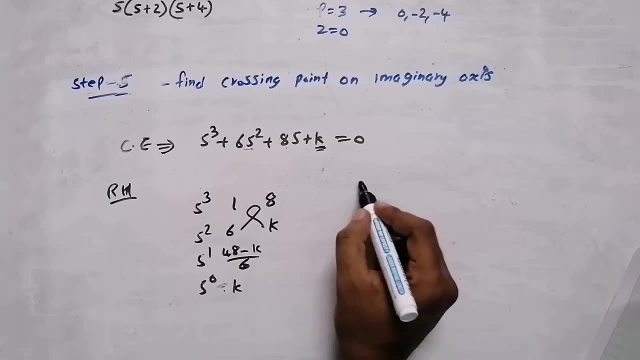 6 into 8, it is 48 minus k divided by 6.. The last value will be our last value, So that is k. Now we need to find the value for k from this point, For finding that 48 minus k divided by 6.. 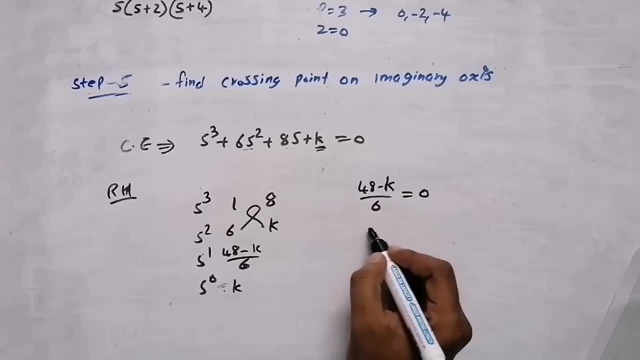 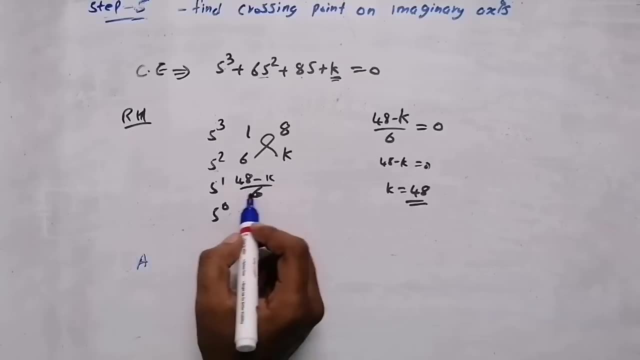 From this we need to find the value of k. Equate that to 0. Then we will get 48 minus k equal to 0.. From that we will get k equal to 48.. Now write the auxiliary equation. So this was our point. when we get 48 minus k by 6.. 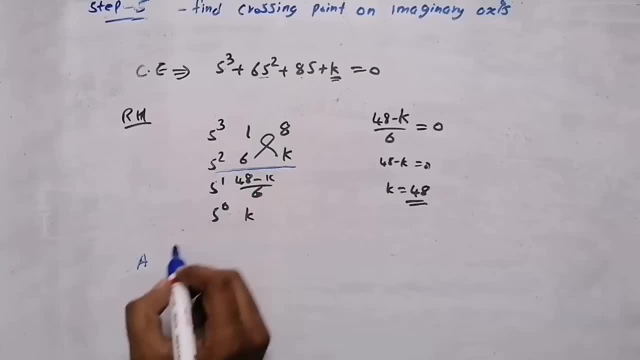 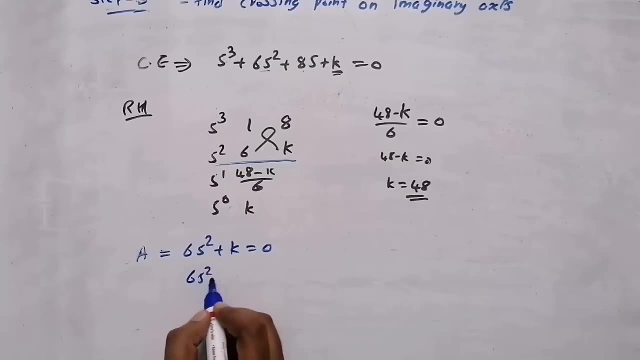 Just above that. Take the equation above that. So the auxiliary equation will be: 6s square plus k, equal to 0.. Now we have the value of k is 41. So 6s square plus 48, equal to 0.. 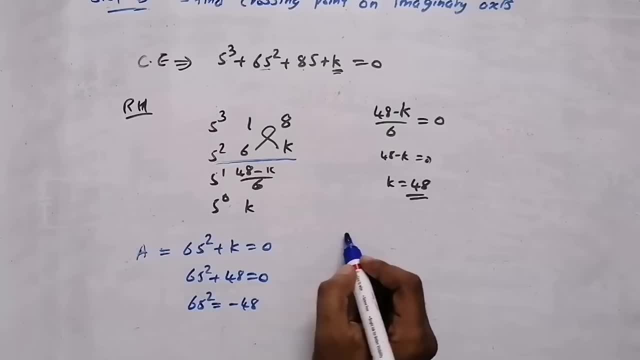 From this we will get 6s square equal to minus 48.. From that, we will get s square equal to 48 by 6.. That will be minus 8.. From this we will get 8s equal to plus or minus root of minus 8.. 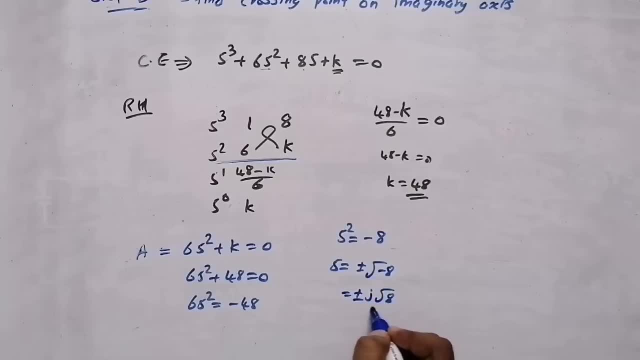 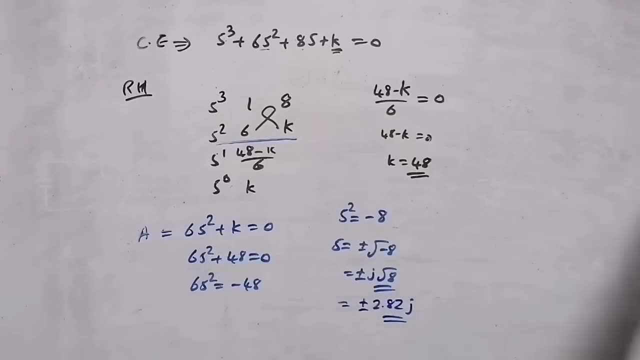 That is plus or minus j root 8.. Okay, Root 8, the value is 2.82.. So plus or minus 2.82.. 2.82j. So plot that point in our graph 2.8.. 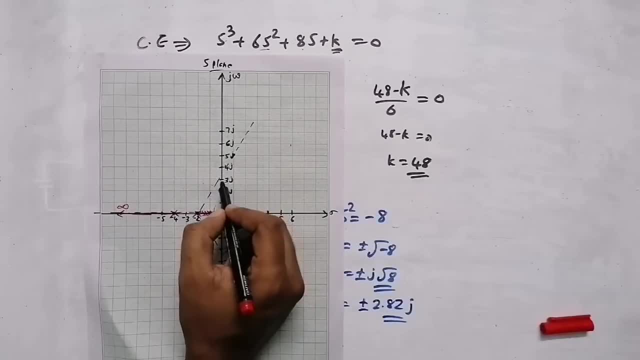 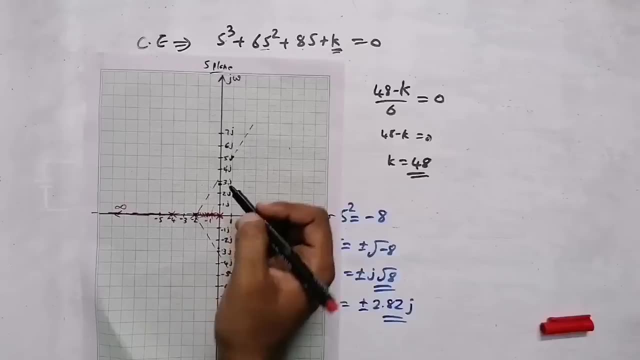 That is 2.8.. 1, 2.. Then this is 3.. So 2.8 will be here, Then minus 2.8.. That is here. So our root locus will be crossing at these two points. 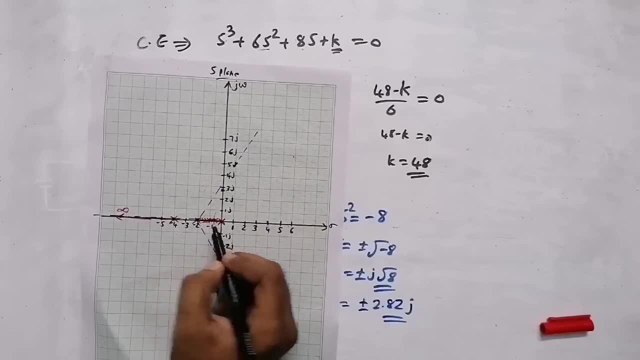 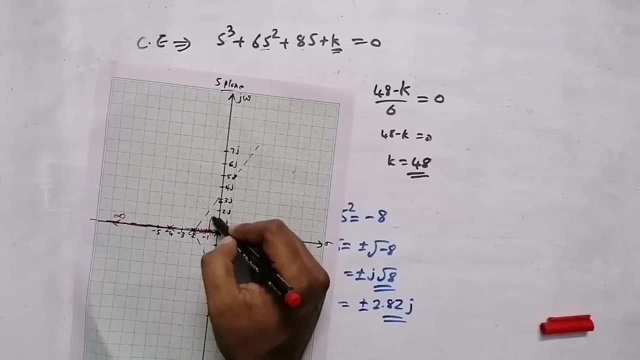 So our root locus will start from pole and it will break away at this point. Then parallel, draw parallel to the asymptote. For that purpose we are drawing asymptote. Our root locus will move parallel to the asymptote, Then it will cross the imaginary axis at 2.82.. 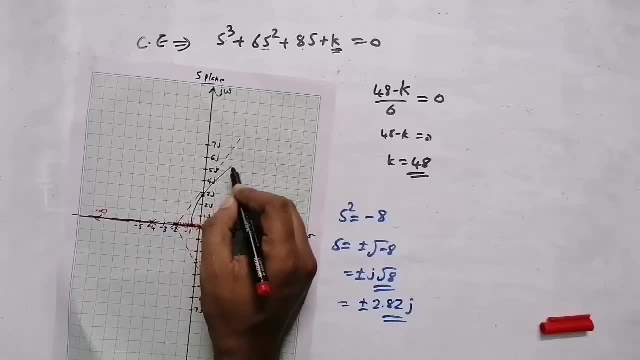 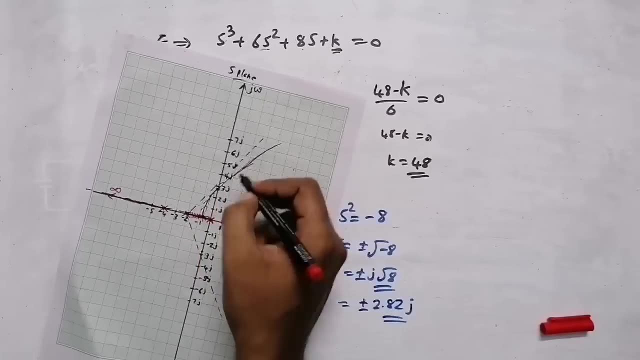 2.82.. Then it will go to infinity. We need to draw parallel to this asymptote. It will go to infinity, So the arrow mark will be starting from pole. The root locus will move like this to infinity. Then in minus side also.